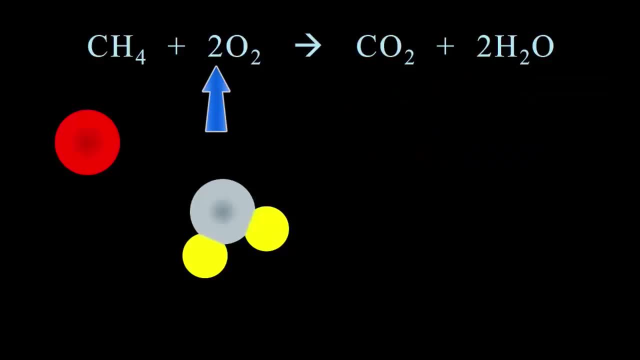 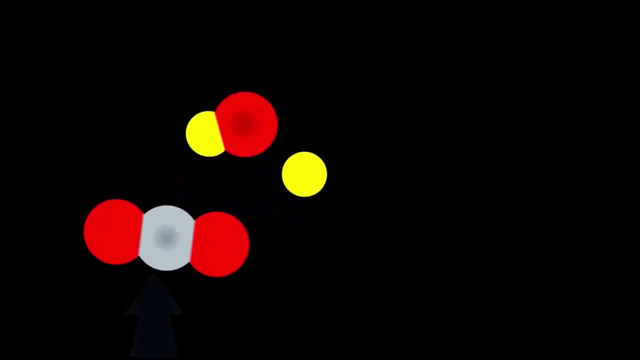 generated. In our balanced equation we had another oxygen molecule, So let's add another one now and see what happens as we watch the reaction proceed. The collisions produce carbon dioxide. What's going to happen next? Two things. When the carbon dioxide forms, it gains a lot of. 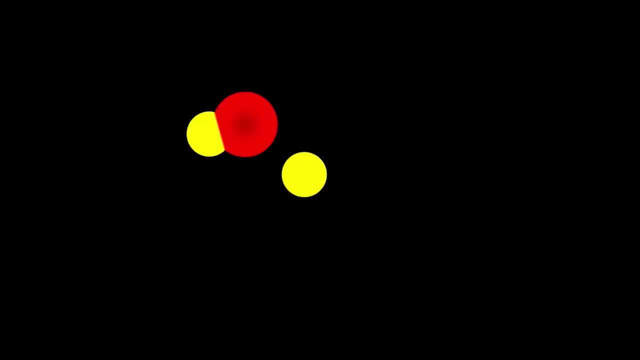 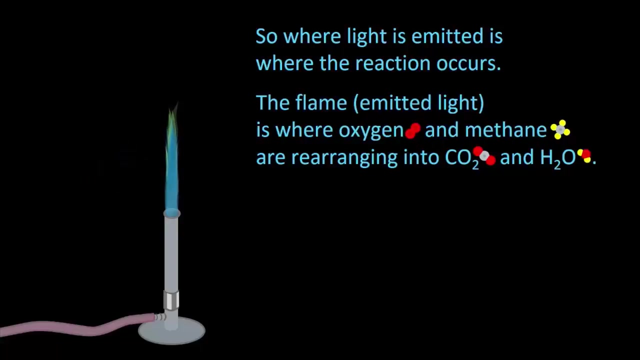 kinetic energy and emits light, And then water again forms at a high kinetic energy and emits light. So where light is emitted is where the reaction occurs. The flame, the emitted light, is where oxygen and methane are rearranging into carbon dioxide and water. The heat we feel is the high kinetic energy. 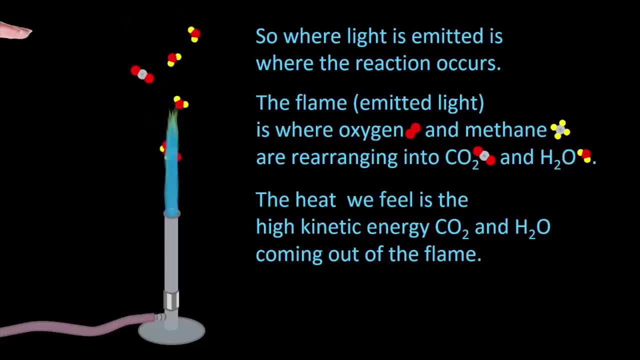 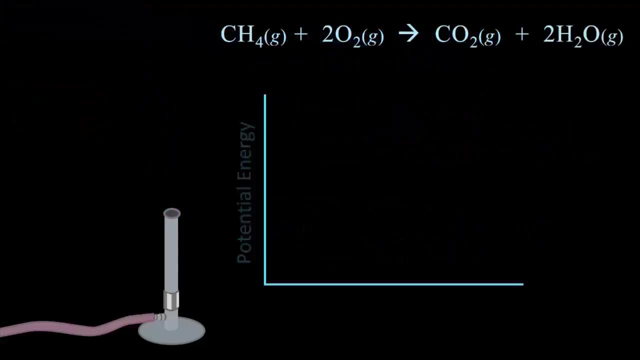 CO2 and H2O coming out of the flame. Our nervous system gets upset when those high speed particles hit our skin, transferring their kinetic energy to the molecules in our skin. Before moving on, let's get a quick summary of what's going on here. We have high potential energy, CH4 and O2,. 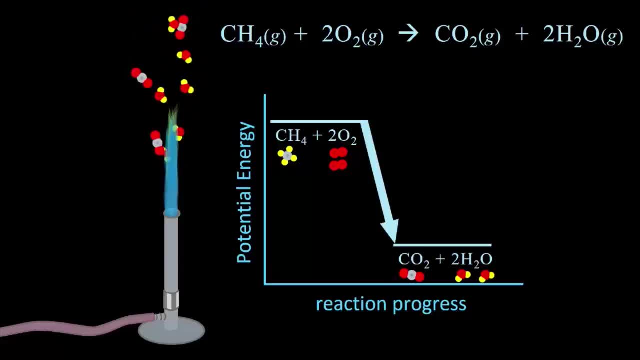 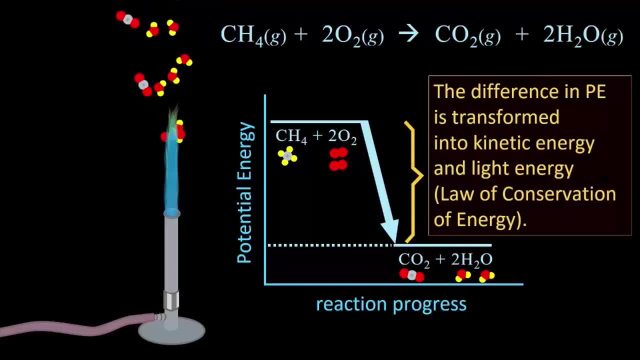 producing low potential energy, CO2 and H2O. That difference in potential energy is transformed into kinetic energy and light energy. The total energy does not change. Our reaction obeys the law of conservation of energy. Let's expand the idea of heat a little bit more. Heat is carried by the 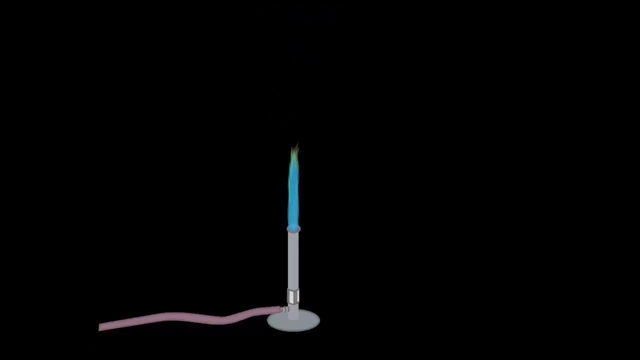 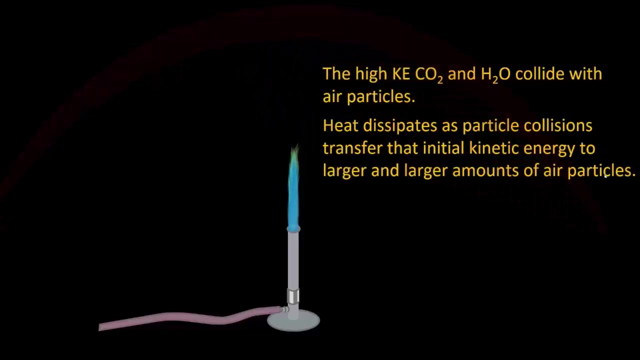 high kinetic energy, water and carbon dioxide. The heat transfers to the air and eventually dissipates. Why does that happen? Well, the high kinetic energy, carbon dioxide and water collide with air particles. Heat dissipates as particle collisions transfer that initial kinetic energy. 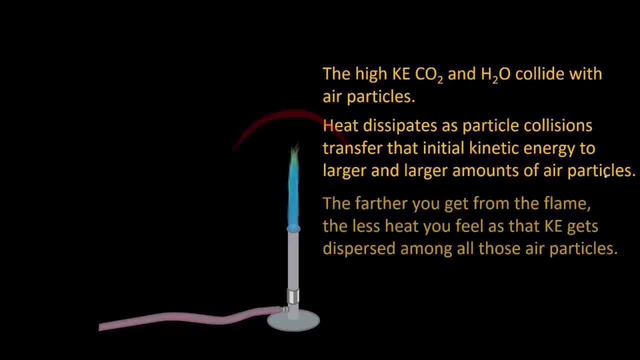 to larger and larger amounts of air particles. The farther you get from the flame, the less heat you feel, as that initial kinetic energy gets dispersed and diluted among all those air particles. Everything we've been talking about here can be applied in general to just about any fire. 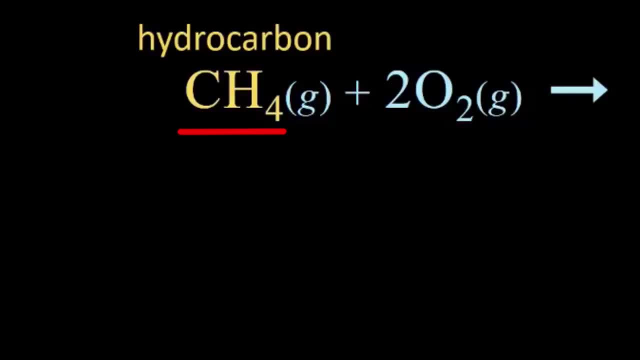 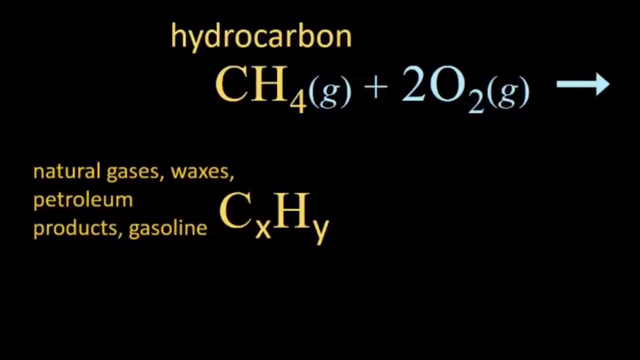 you encounter. CH4 is what is called hydrocarbon, and hydrocarbons provide the fuel for almost any fire you might see. Hydrocarbons are any compounds made out of carbon and hydrogen. There are many, many hydrocarbons that we encounter, such as natural gas, and methane is the 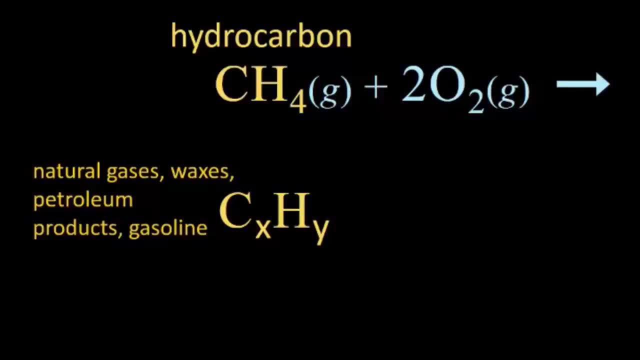 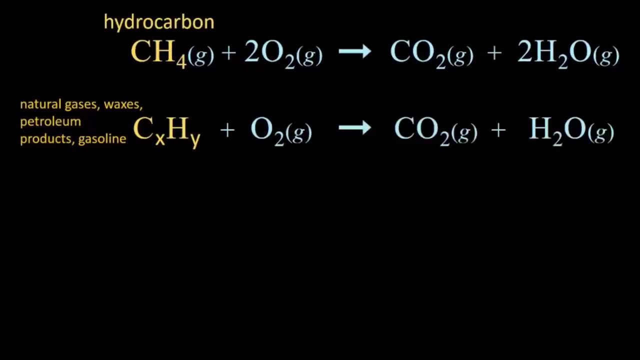 largest component of natural gas. so that's what you see burning on your stove, as well as waxes, petroleum products such as gasoline. When you burn them, they produce carbon dioxide and water and light. Hydrocarbons can also be somewhat oxidized, including carbohydrates and lignan, which 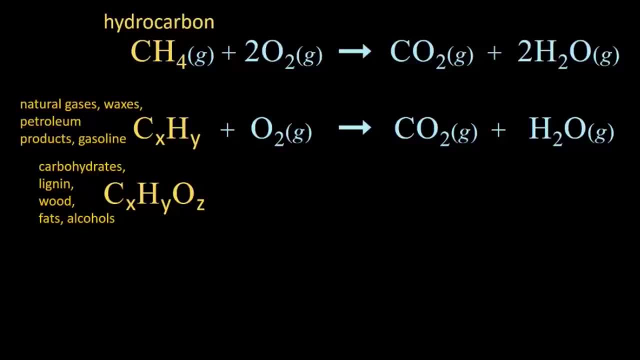 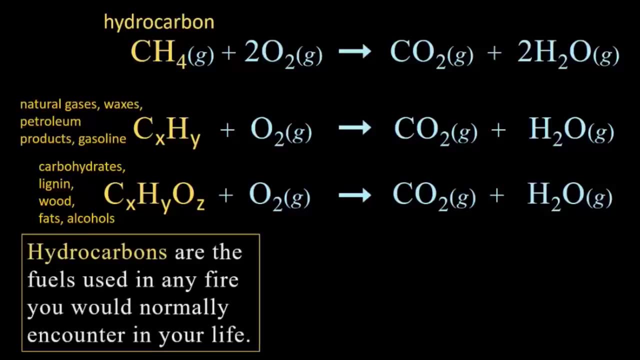 incidentally, are the two major components of wood. There are also fats and alcohols and when you burn them you produce carbon dioxide and water and light. Hydrocarbons are the fuels used in any fire you would normally encounter in your life. The formation. 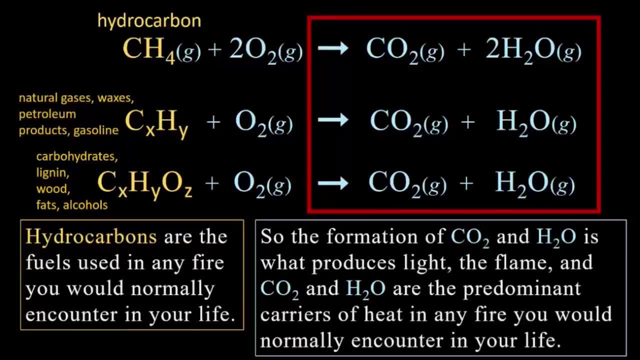 and water is what produces light, which is the flame, and carbon dioxide and water are the predominant carriers of heat in any fire you would normally encounter in your life. And that is the story of fire. 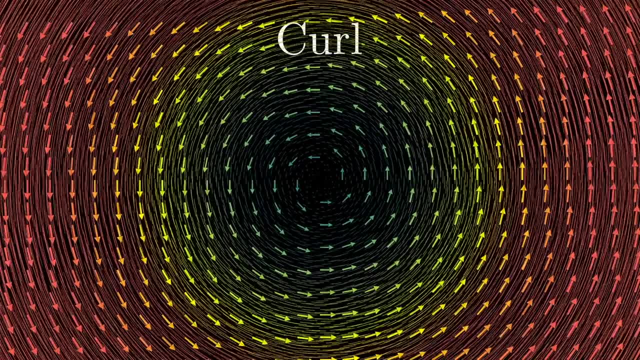 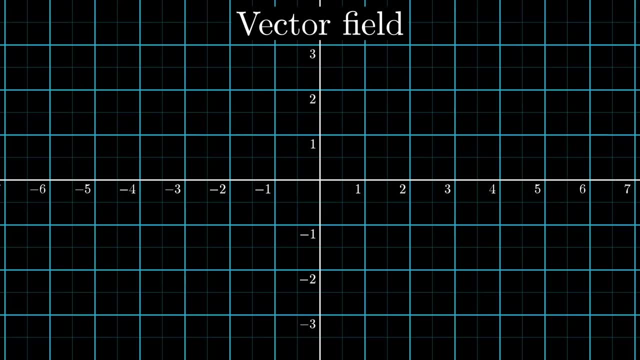 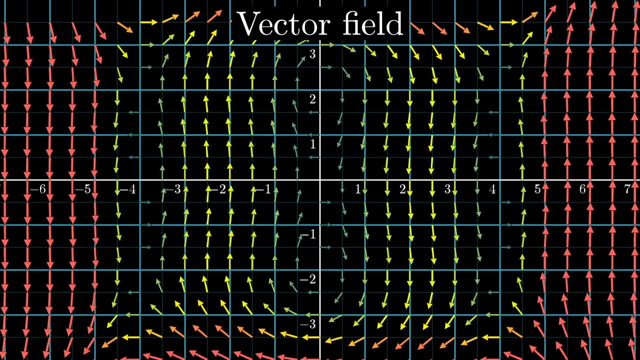 Today, you and I are going to get into divergence and curl. To make sure we're all on the same page, let's begin by talking about vector fields. Essentially, a vector field is what you get if you associate each point in space with a vector- some magnitude and direction. Maybe those vectors represent the velocities. 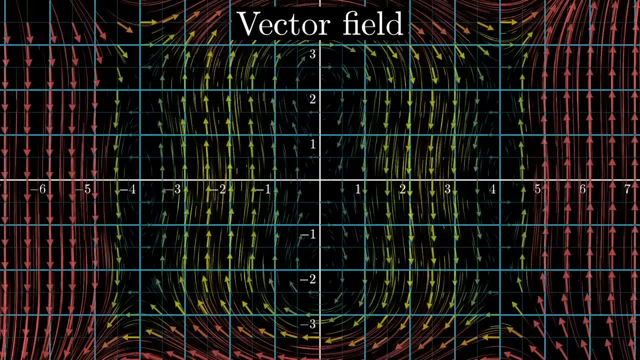 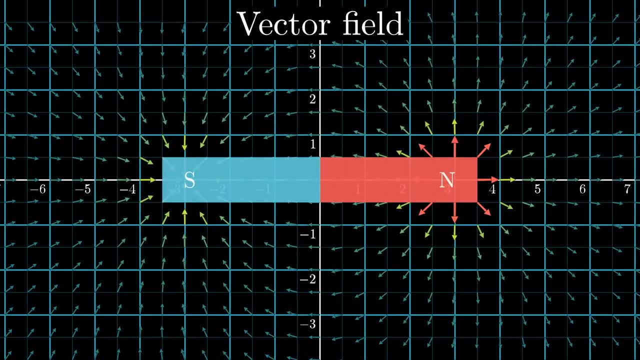 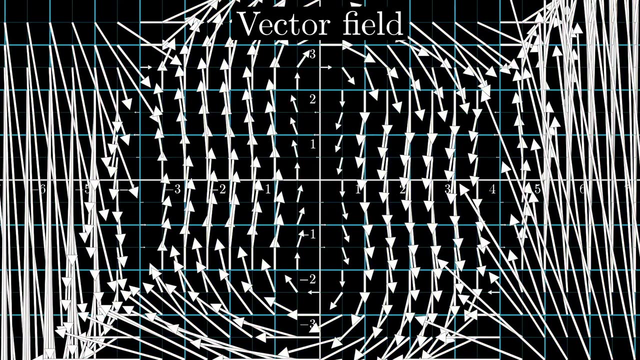 of particles of fluid at each point in space, or maybe they represent the force of gravity at many points, or maybe a magnetic field strength. Often, if you were to draw vectors to scale, the longer ones end up just cluttering up the whole thing. It's common to lie a little or artificially shorten ones that are too long. 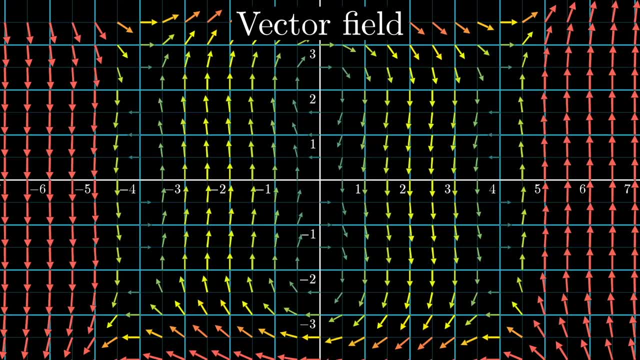 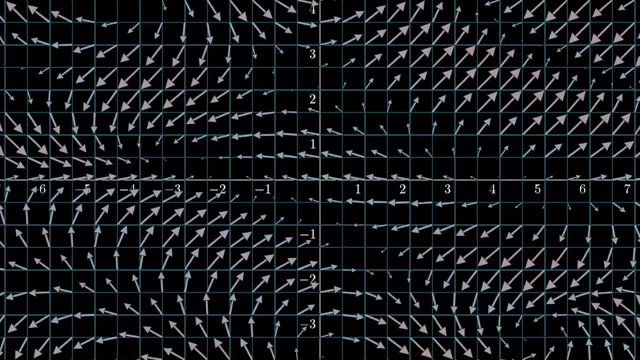 maybe using colour to give some vague sense of length. In principle, vector fields in physics might change over time In almost all real-world fluid flow. the velocities of particles in a given region of space will change over time. In principle, vector fields in physics might change over time In almost 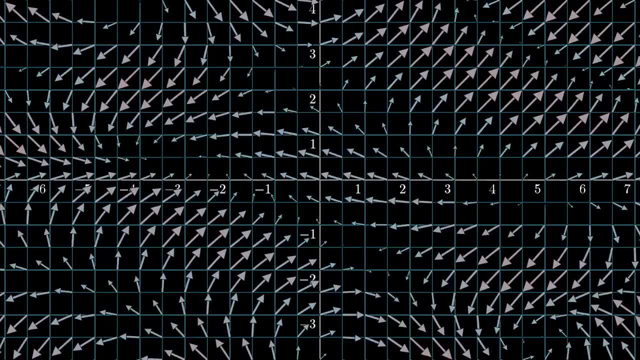 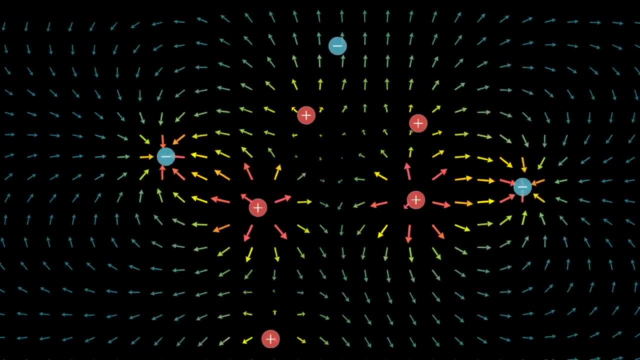 over time. In almost all real-world fluid flow, the velocities of particles in a given region of over time in response to the surrounding context. Wind is not a constant. it comes in gusts and electric field changes as the charged particles characterizing it move around.